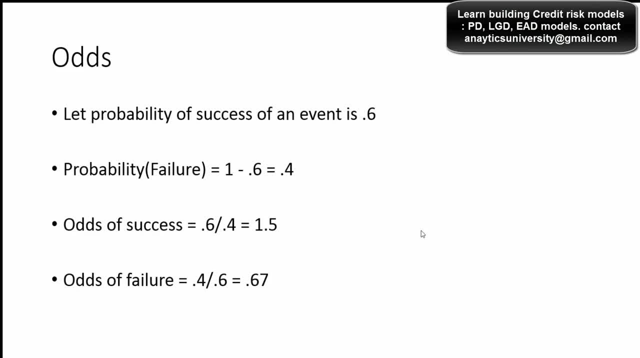 odds of success equal to the probability of success by probability of failure. 0.6 by 0.4, equal to 1.5.. So what is the probability of, or the odds of failure? Odds of failure equal to the probability of failure divided by the probability of success. So it's the reciprocal. 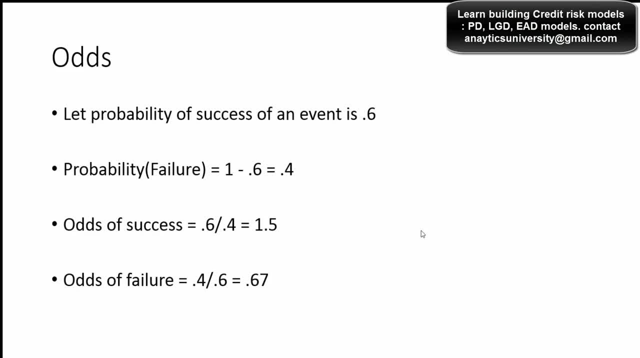 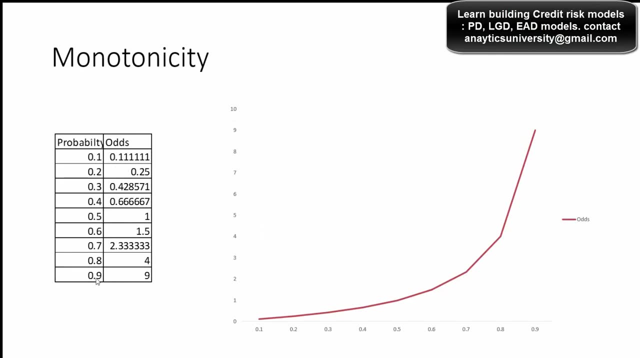 of odds of success: 0.4 by 0.6, equal to 0.67.. So that's how we define the odds of success and odds of failure. What I have done here is that, for each probability ranging from 0.1 to 0.9, I have calculated what is the odds of success And you can see in the graph. 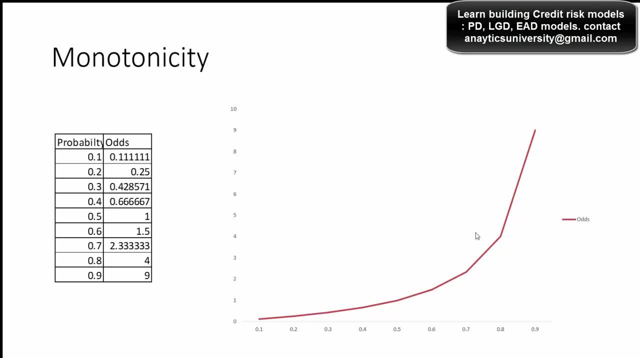 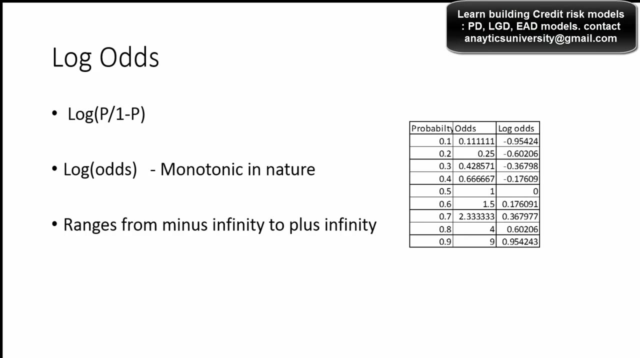 it's increasing in nature, So it's monotonous in nature. As the probability increases, it goes up, and it also goes up right. It ranges from 0 to the positive plus infinity. What is log odds? Well, log odds is nothing but the logarithm of odds. If p is the probability, 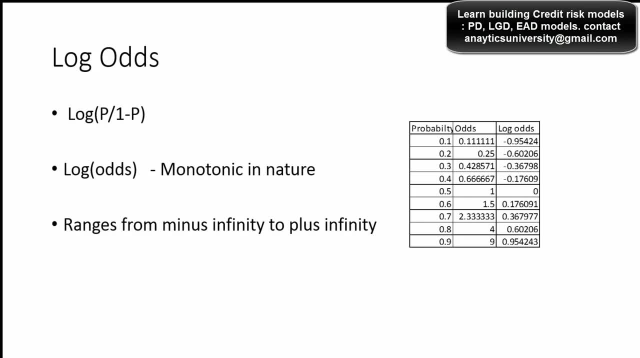 of success and 1 minus p is the probability of failure. then we define log odds as log of p by 1 minus p, as you can see on the screen. Like odds, log odds also follow the monotonicity, That is, with increase in the probability. 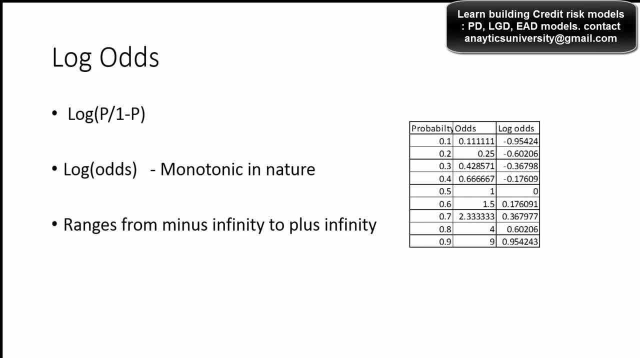 the log of values also increases. The log odds ranges from minus infinity to the plus infinity. You can see on the screen I have probability values ranging from 0.1 to 0.9.. And the corresponding odds and log odds. What is the importance of log odds with regards? 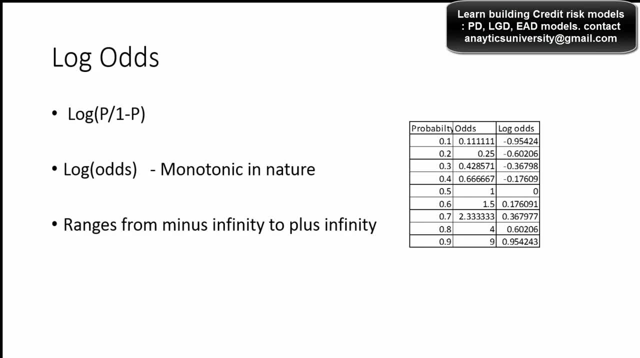 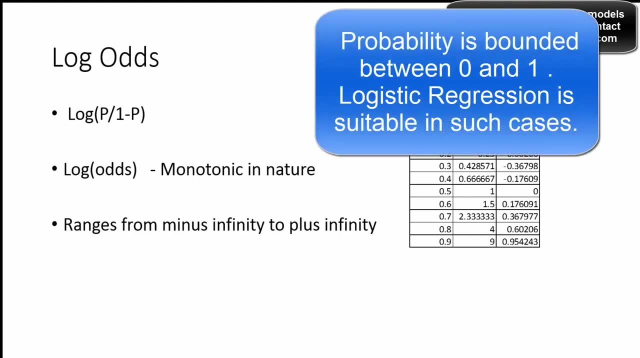 to logistic regression. Well, it's very important. Why don't we just model for the probability directly? Why do we model the log odds of the probability? As you know, probability ranges from 0 to 1.. So it's a bounded value. The upper bound is 1,. the lower bound is 2,. 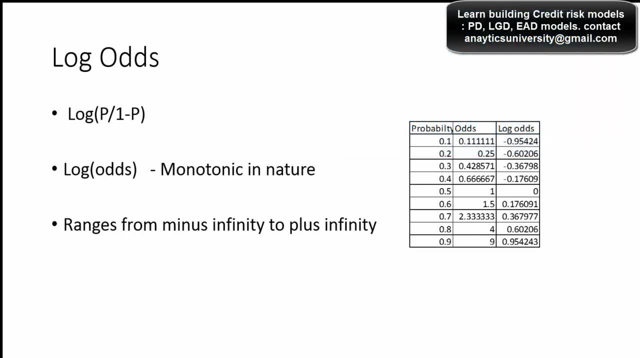 and the lower bound is 0. It's very difficult to model such a variable. We take the logarithmic transformation of the odd and then model, So it serves two purposes. One of the good things for us is that log odd is not bounded. It ranges from negative infinity minus infinity. 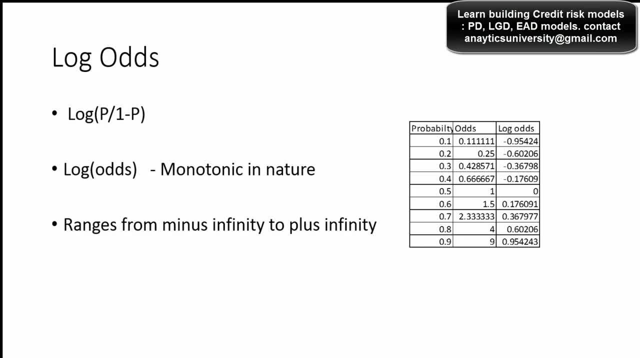 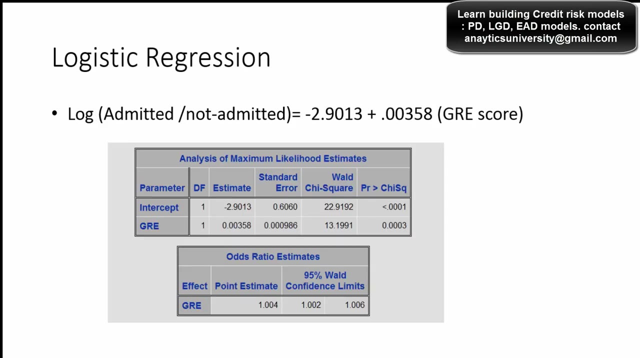 to plus infinity, And then it's a very simple transformation. It can be explained very easily. So these are the two reasons why we actually model log odds instead of the actual probability value in logistic regression. To explain how to interpret the odds ratio, I have taken 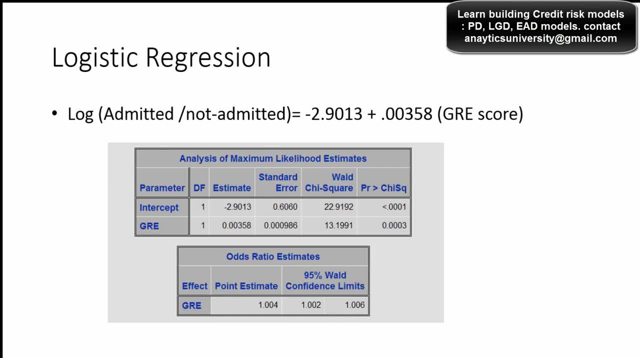 a very simple example here. Well, this is directly a model coming from a computer. This is a model coming from one of my data sets, wherein the dependent variable is admit, whether a student is admitted to a graduate school or not. So if a student is admitted, 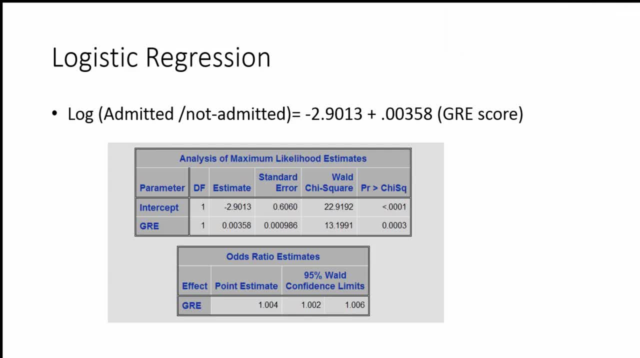 the dependent variable takes 1, else it takes 0. So it's a binary variable. I have used logistic regression to model this variable. I have got one independent variable, which is gre score. My model looks like this: Log of admitted by not admitted, just like p by. 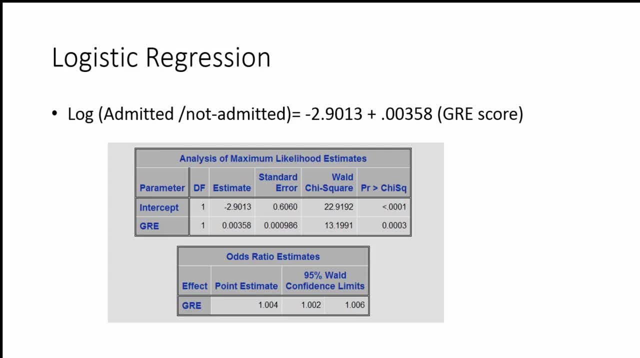 1 minus p right is equal to minus 2.9, which is the intercept plus 0.00358 gre score. So 0.00358 is my slope coefficient for gre score. You can see that in the analysis of. 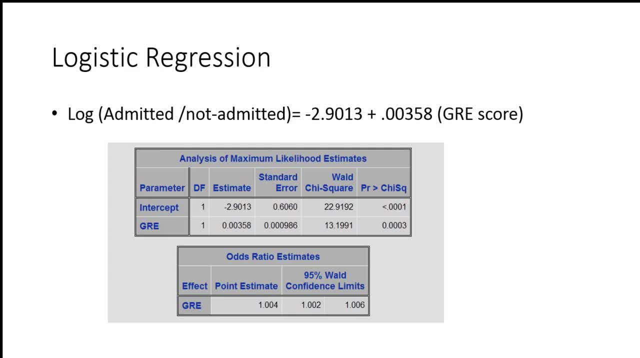 maximum likelihood estimate. you know this is directly taken from the SAS output. You can also see the odds ratio estimates. for the independent variable It's 1.004.. So we are curious to know how odd ratio is interpreted and how is it related to the maximum likelihood? 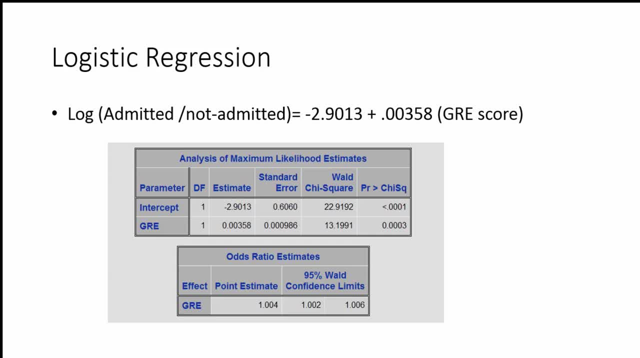 estimates. So before I you know talk about the mathematical explanation, let me let me tell you that odd ratio is nothing but the exponential of the maximum likelihood estimate. But how do we know that, that it's the exponential of maximum likelihood estimate? Okay, we will. 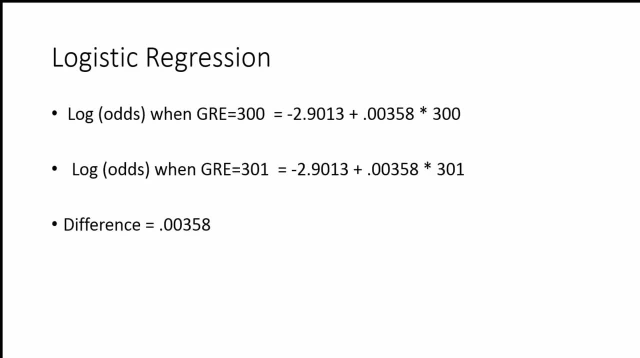 see. why is that so? Let's assume that a student has a gre score equal to 300. So what is the log odd that that particular student will get admitted to the graduate school? Well, put 300 in place of in place of the variable gre and calculate the log odd Minus 2.9 plus. 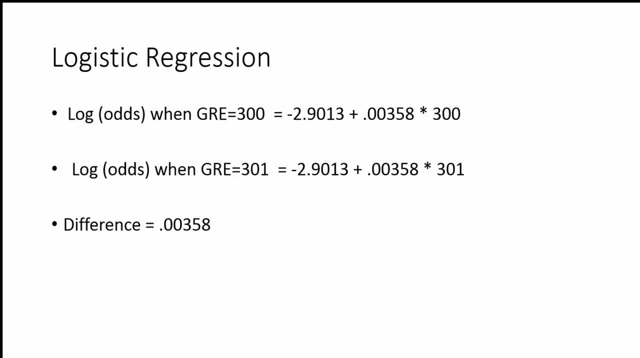 0.00358 into 300.. That the gre score increased by 1 unit. Now the gre score is 301.. So what is the log odd? Use the same equation, same, you know, logistic regression equation In place of 300, you. 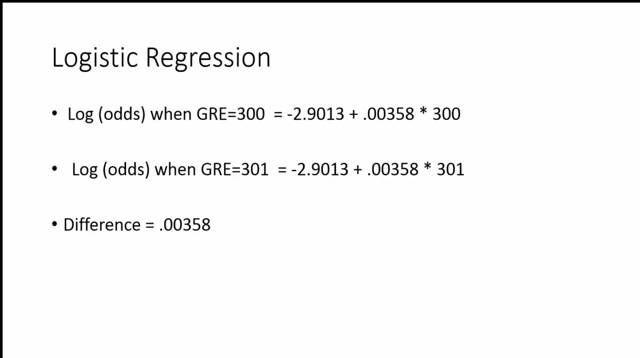 just put 301 this time. Okay, So what is the difference between the log odds when the gre score increases by 1 unit? Well, you just, you know, subtract one from the other. We will subtract the second equation from the first, and it can be done very easily. So what? 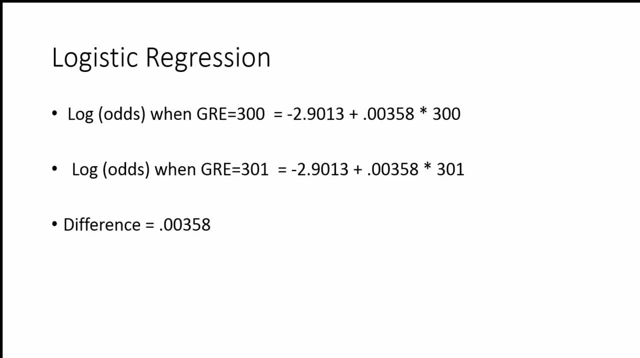 is the difference? The difference in the log odds is nothing but 0.00358.. So is this number familiar? Yes, it is. So what is 0.00358?? This number is nothing but the slope coefficient of gre. Okay. 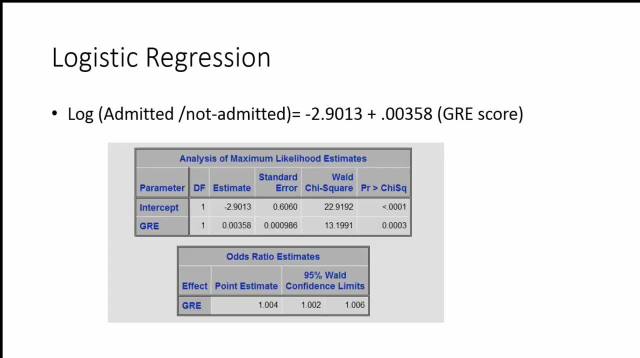 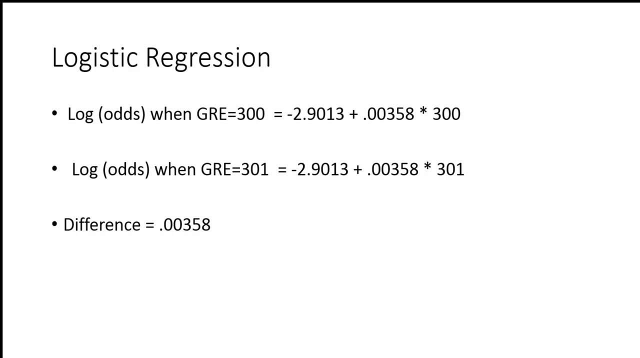 Okay, If you go back and see what is the slope coefficient or what is the estimate for gre, it's the same number, 0.00358.. When there is a unit change in the independent variable, the corresponding change in the log odd is nothing but the estimate of that particular. 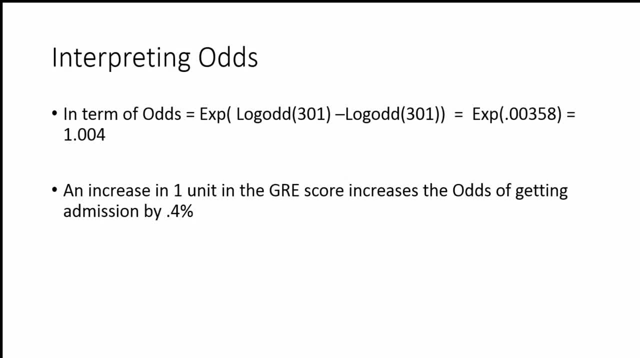 independent variable. So what has it to do with log odd? Okay, We saw that. how to interpret the log odds? It's nothing. but you know, the change in log odds is nothing but estimate itself. Let's transform this in terms of odds. In terms of odds, we just need to take: 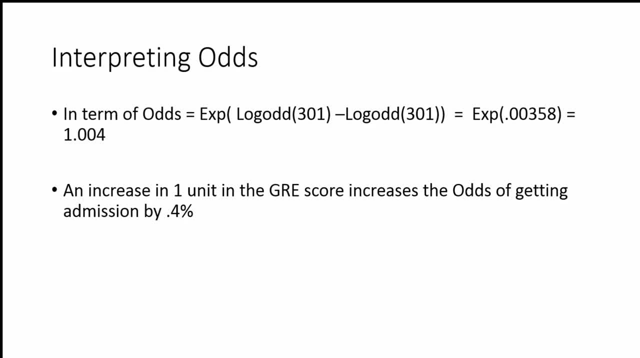 the exponential of that. You know that the reverse transformation of logarithm is nothing but the exponential. If you take the exponential of the difference of log odd, okay, you can see on the screen. you just have to take the exponential of 0.00358.. Okay, Because 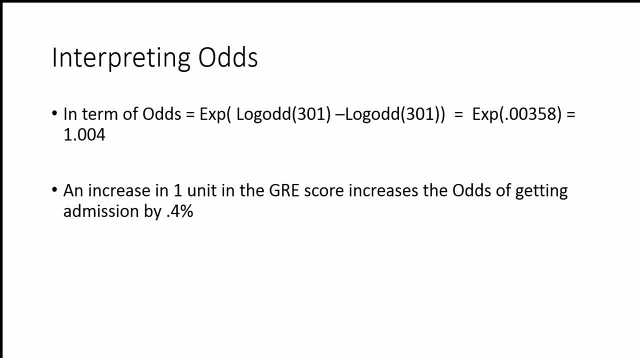 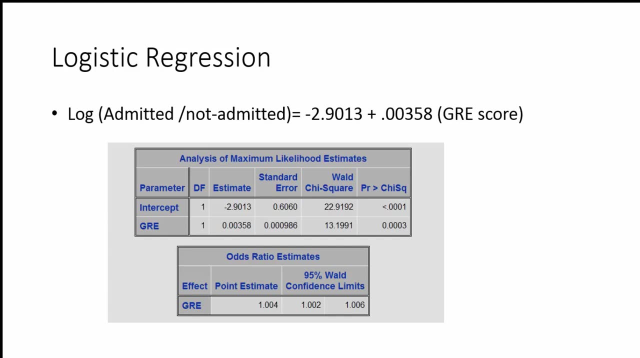 that is the difference between the log odd, which comes out to be 1.004.. Okay, So what is 1.004?? Let's go back and check if this figure is you know, this figure or this number appears in our output. Well, 1.004 is nothing but the odd ratio. estimate of gre, The exponential. 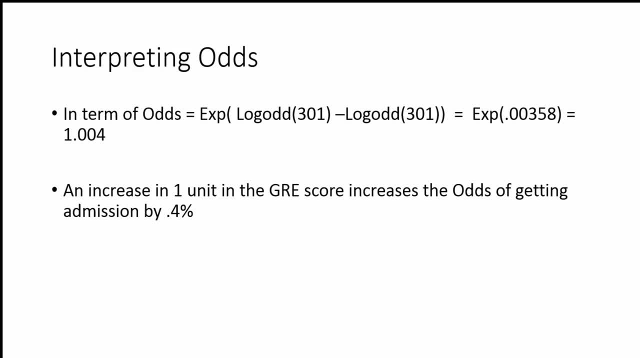 of the change in the log odds. Okay, Okay. So odd ratio is nothing but the exponential of the change in, or the difference in, log odds. So how do we interpret it? How do we interpret the odd ratio? Well, an increase in one unit in the GRE score increases the odd of getting admission in the graduate school. 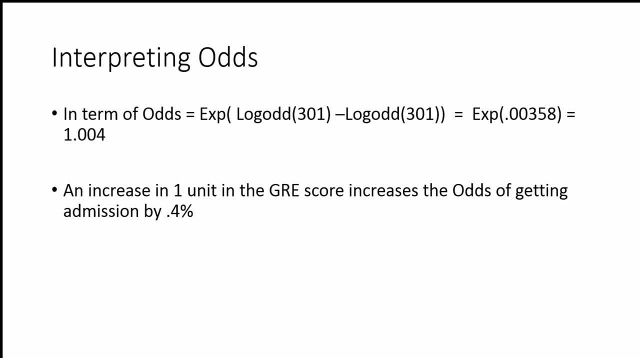 by 0.4%. Why does this 0.4% come from? Well, you can see 1.004.. Okay, So the extra value you know after the one is what is added to the you know chances of getting admitted one from. 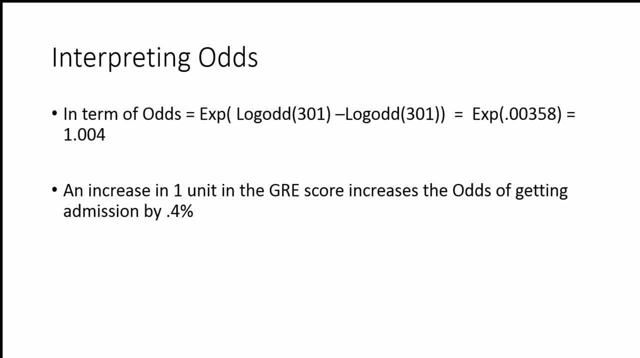 there. So what remains is 0.004.. Had it been 2.004, just subtract one, it remains 1.004.. Right, So, and change it to percentage. change it to in terms of percentage. Okay, So 0.004. 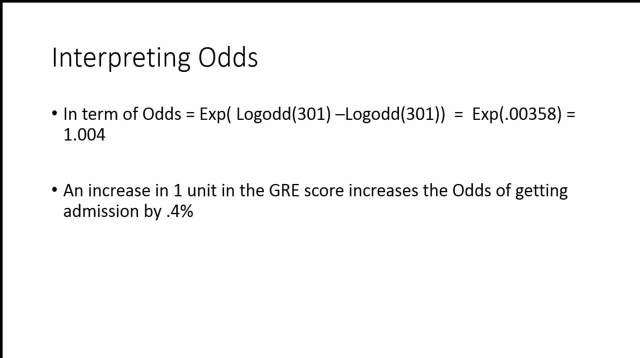 in percentage terms it's 0.4%. So an increase in one unit in the GRE score increases the odds of getting admission in the graduate school by 0.4%. So that's how we interpret the odd ratio in a logistic regression. Thank you.